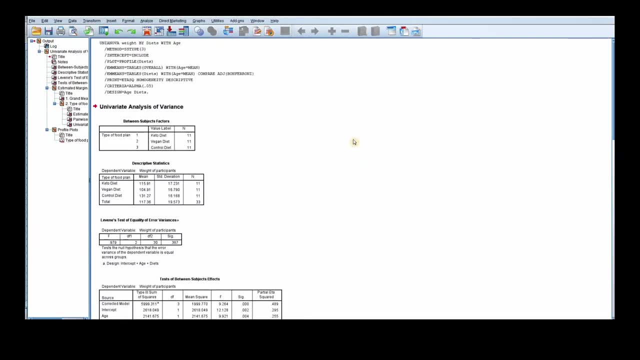 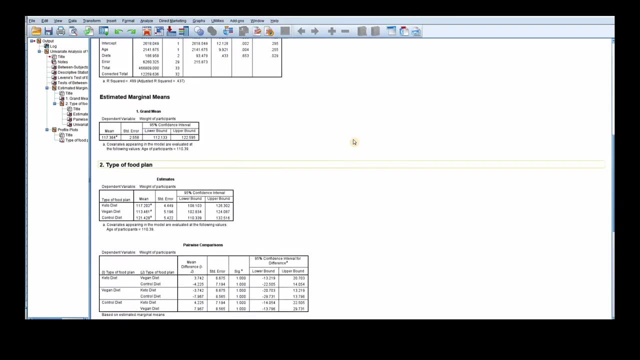 to get these types of results and the procedure you should take to enter the raw data into XPSS for the data analysis are two important things that have been fully demonstrated in this video, So I strongly encourage you to see this video to the end in order to learn. 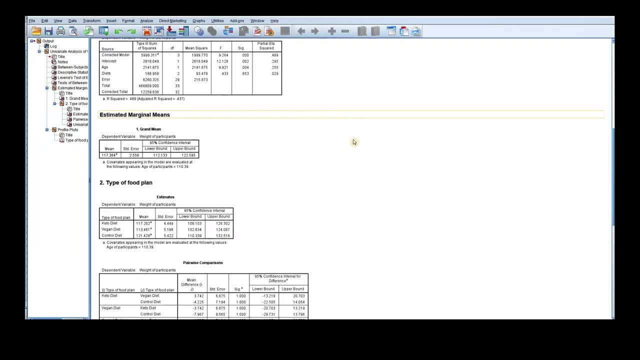 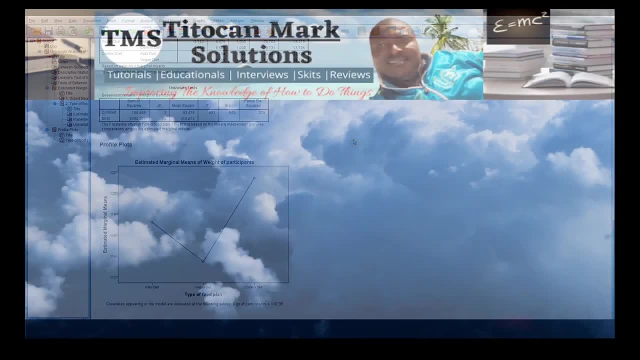 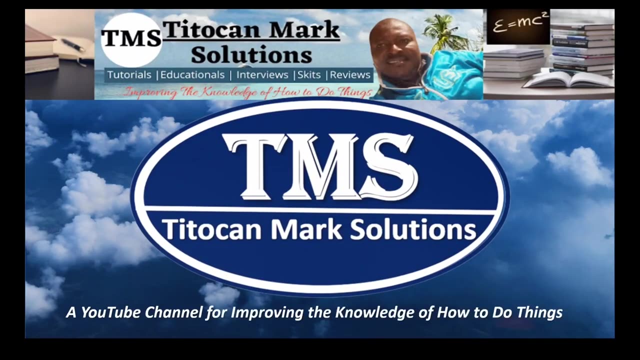 the best way to perform ANCOVA analysis in XPSS. But before I go into the demonstrations in XPSS, let me quickly give you the synopsis. My name is T-Token and this is T-Token Max Solutions, a YouTube channel for improving the knowledge of how to do things One-way. 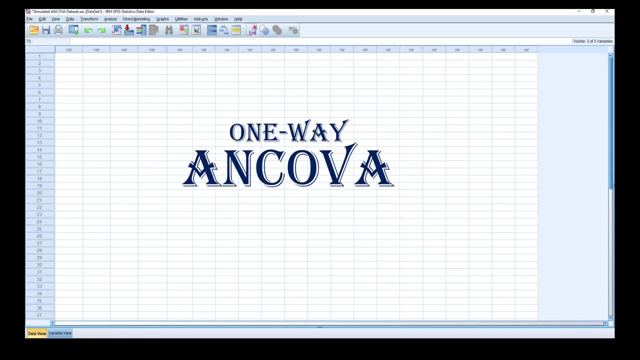 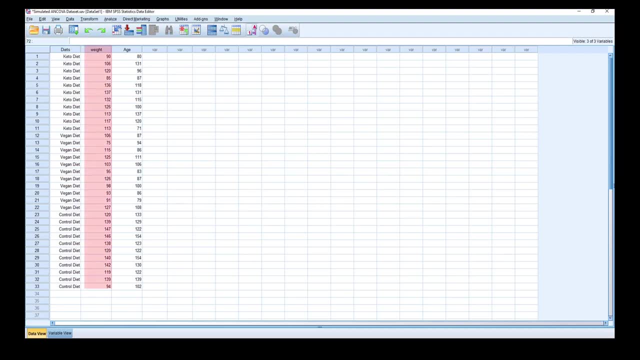 analysis of covariance, or simply put one-way. ANCOVA is a statistical technique used to measure the value of the data in XPSS. It is used to compare the means of a continuous dependent variable across two or more groups of an independent variable, while statistically controlling for the effect of one or more. 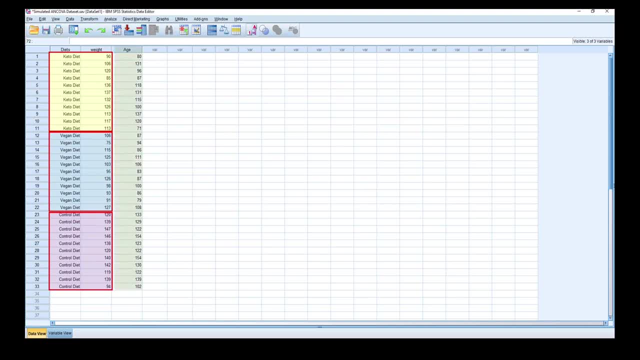 continuous independent variables, known as covariates. Technically, ANCOVA extends the analysis of variance or ANOVA, by incorporating the influence of covariates. This technical extension provided by ANCOVA allows for a more accurate assessment of group differences. 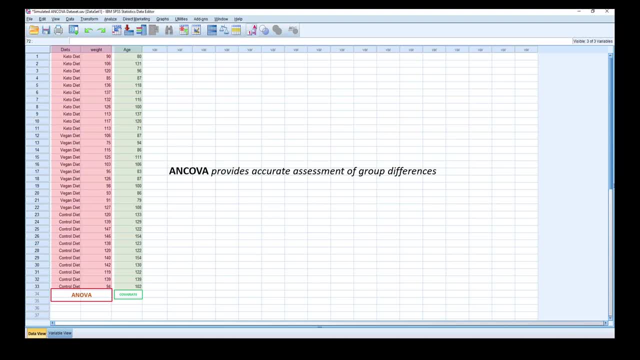 There is also the incorporation of regression principle in ANCOVA, but I will be silent on that in this demonstration. Basically for a one-way ANCOVA analysis in XPSS, your table of raw data sets should take the following structure: There should be one nominal or. 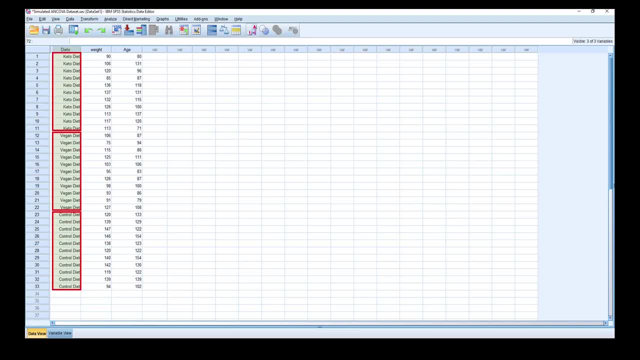 categorical independent variable, which should have two or more levels or groups. There should be one continuous dependent variable, which is the variable of interest, And there should also be one continuous dependent variable which is the variable of interest, And there should also be one or more continuous covariate variables, also called confounding factors. 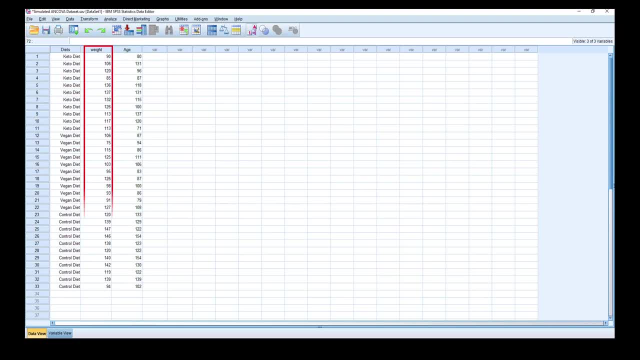 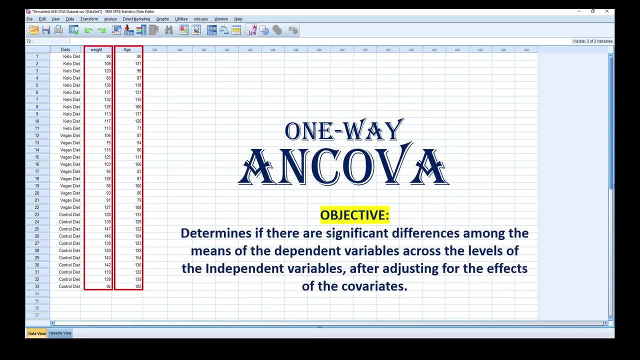 As you can see from this table of raw data sets, there is only one variable of interest, which is my dependent variable, and at least one covariate variable in my data set. This is why this analysis is called one-way ANCOVA. The objective of performing ANCOVA is to determine: 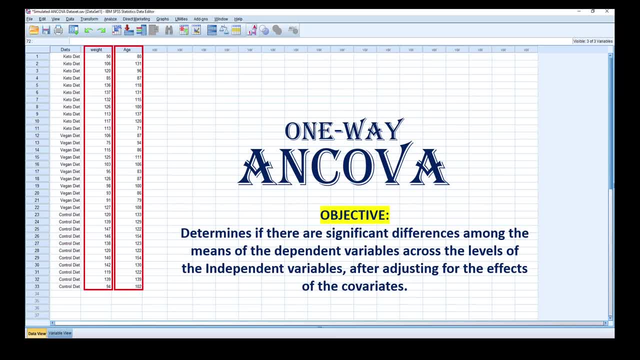 whether there are statistical differences in the means of the dependent variables across the levels of the independent variables, after adjusting for the effect of the covariates. For you to be able to successfully run the ANCOVA analysis in XPSS and have valid results, 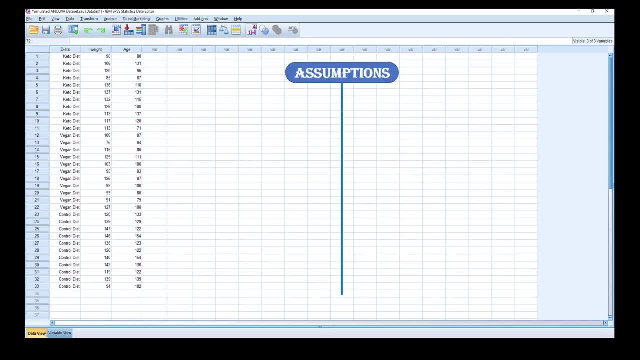 your data set must satisfy the following assumptions as parametric conditions that must be met for ANCOVA. But you must know that if you fail to test your data for the assumptions, XPSS will still produce some results for you, but such results will not be valid. outcome of. 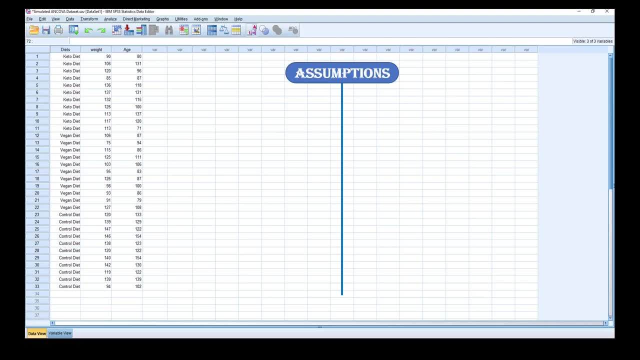 what are expected. so it's important that you ensure your set of data satisfy the parametric conditions for one-way ANCOVA. The assumptions are: 1. Your dependent variable and covariate variables should be measured on a continuous scale, That is, they should be measured at the interval or ratio level. This can be verified by visual. 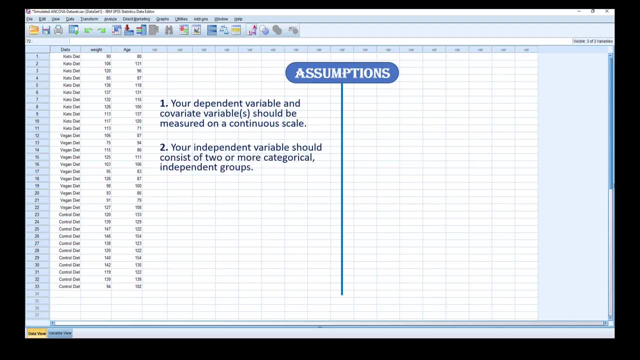 inspection 2.. Your independent variable should consist of 2 or more categorical independent variables groups. Example of independent variables that meet this criteria is gender, which is just two groups, that is, male and female. Another example is ethnicity in Nigeria, which is five groups in. 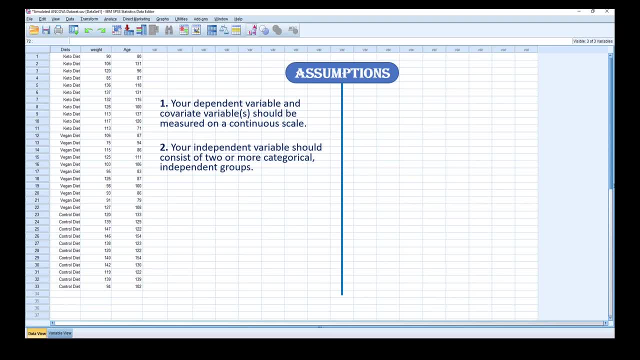 this case, that is, Igbo, Hausa, Yoruba, Isha and Orobo. These assumptions can be verified by visual expression too. Three: your data should have independence of observations. This means that there should be no relationship between the observations in each group or between the groups. 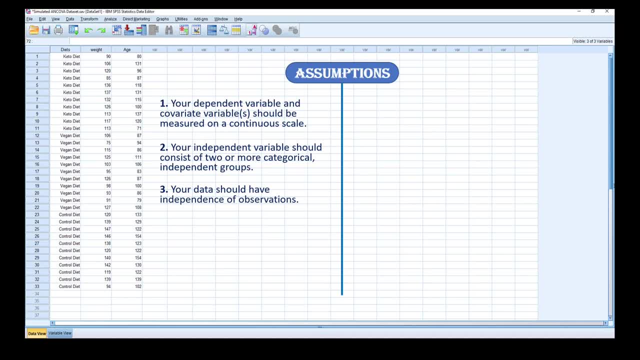 themselves. That is, there must be different participants in each group, with no participant being in more than one group. This can be tested by visual expression or, more preferably, using W Watson test statistics Four. there should be no significant outliers in your data set. 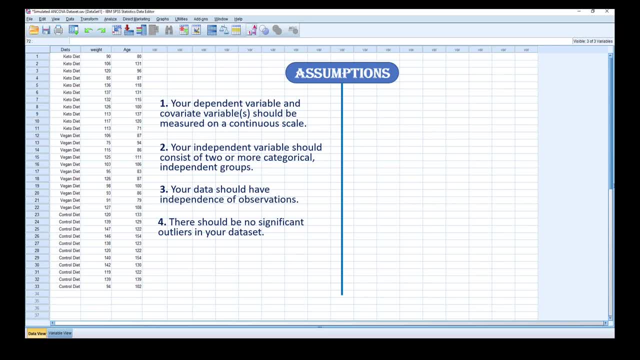 Outliers can create problems when they are present in your data, because they can create a negative effect and reduce the validity of your results. One of the simplest ways to test for this assumption is to use a bus plot Five. your residuals should be approximately normally distributed for each. 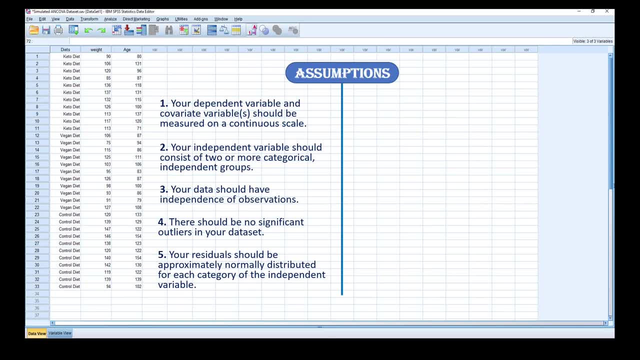 category of the independent variable. You should test for normality using Shapiro weak test of normality. Want to test for within group residual And want to test for overall model fit Six. there needs to be homogeneity of variances, That is, there must be equal variances across your data set. You can test this assumption. 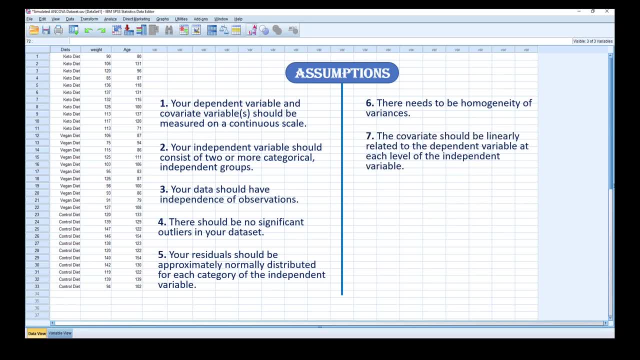 using Levens test statistics Seven. the covariance should be linearly related to the dependent variable at each level of the independent variable. You can test this assumption by plotting the grouped scatterplot of the covariance post-test scores of the dependent variable and independent variable. 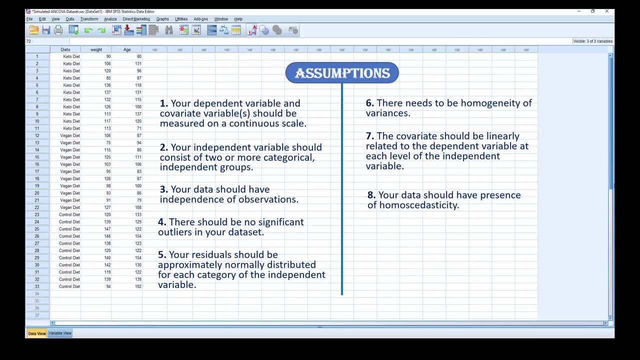 8. Your data should have presence of homoscedasticity. You can test this assumption by plotting scatterplot of the standardized residual against the predicted value. And 9. There should be homogeneity of regression slopes, which means that there is no interaction. 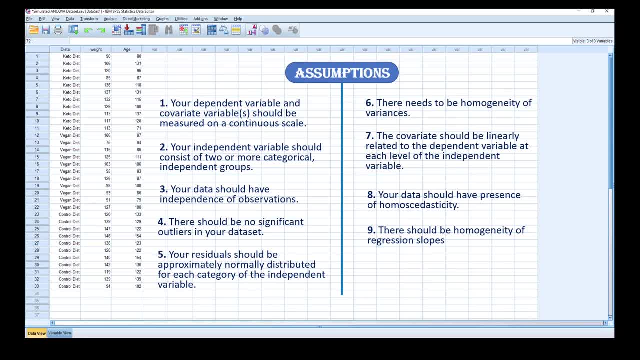 between the covariant and the independent variable. Please note that if you do not run the statistical test on these assumptions correctly, the results you get when running a one-way ANCOVA may not be valid. So the onus is on you to ensure that the data you are running for ANCOVA is tenable for. 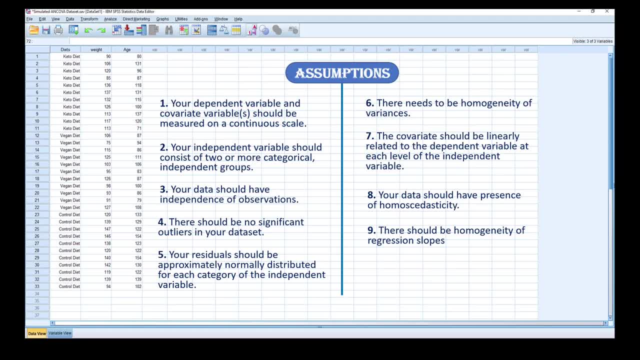 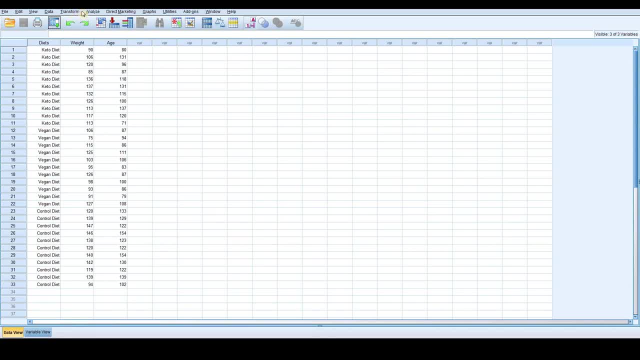 the analysis. Now let me go into XPSS and demonstrate the statistical procedure to perform analysis of covariants. Go to the menu bar and click on Analyze. From the submenu, put your cursor on General Linear Model and from these drop-down options, 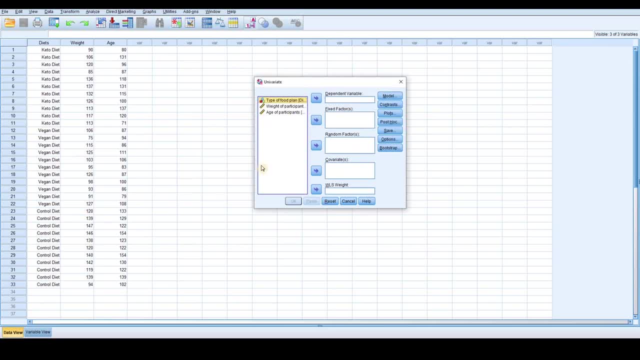 click on Univariant and this opens the Univariant dialog box. As you can see in this dialog box, your variables are in the box on the left But, as you can see, the variable names are represented by their labels. I would like to use their variable names instead. 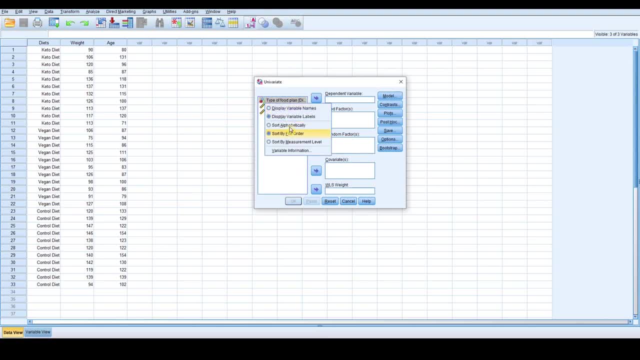 So right-click on any of the labels in the box on the left and, from the options that pop up, click on the radio button for Display Variable Names to display the true variable names. These include the diet, the weight and the age. Now click on the weight and the age. 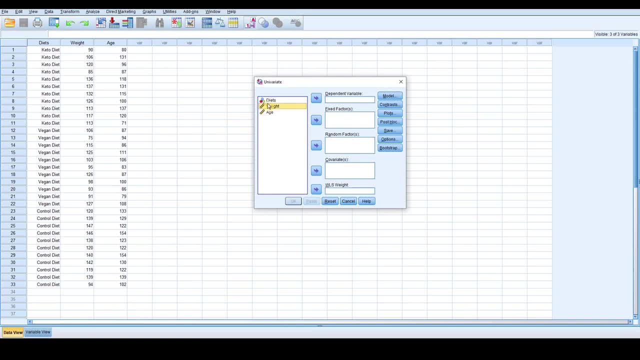 Now click on the weight and the age. Next, click on the weight, which is my dependent variable, and click on this transfer arrow key to move it to the dependent variable box. Then click on the diet, which is my independent variable, and use this transfer arrow key to. 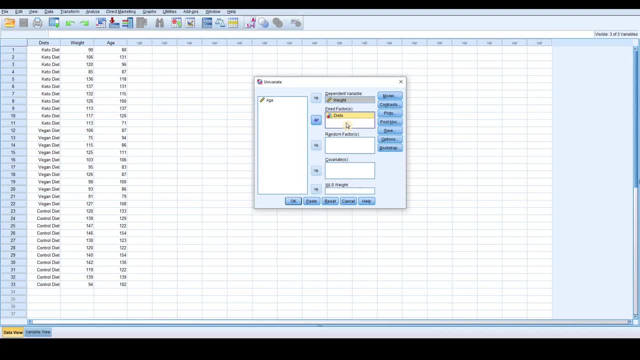 move it to the feast factor box. The next variable to move is the age, which is my covariant or conf boundary factor. Click on the age and transfer it to the covariant box. Now click on the Model button to open the Model dialog box. 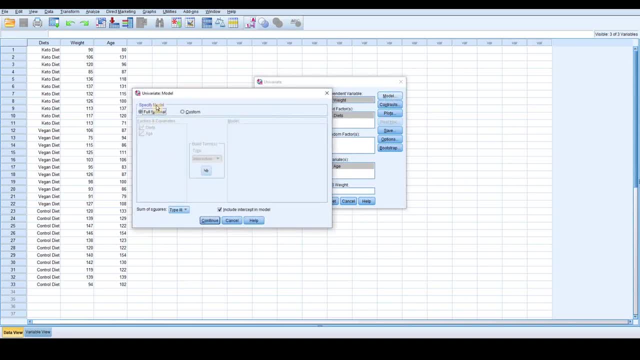 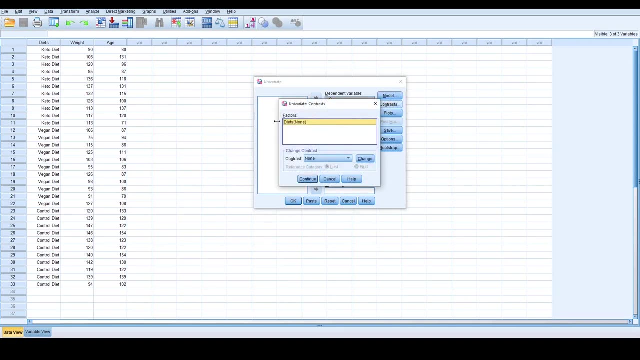 Now method 3s In this dialog box. ensure that the default specified model selection is full factorial and the sums of square is type 3.. Click continue to close this dialog box. The next button is contrast. For this demonstration, I don't intend to change the contrast, so leave the default contrast. 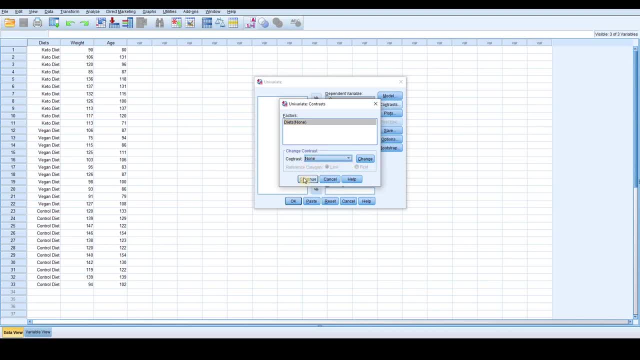 selection as none and click continue to close this dialog box. Now open the plot button In this dialog box. the only factor available in the box on the left is diet, So click on this transfer arrow key to transfer it to the horizontal as is box. 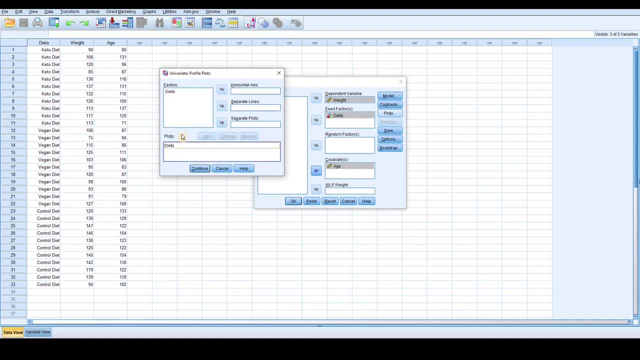 Thereafter click add to add the diet variable to what should be plotted by the uncover function. Then click continue to close this dialog box. The next button to open is save. Do not check any box here, as doing so will not affect the uncover result. 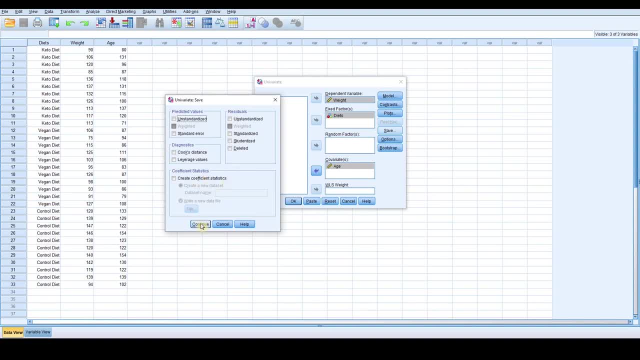 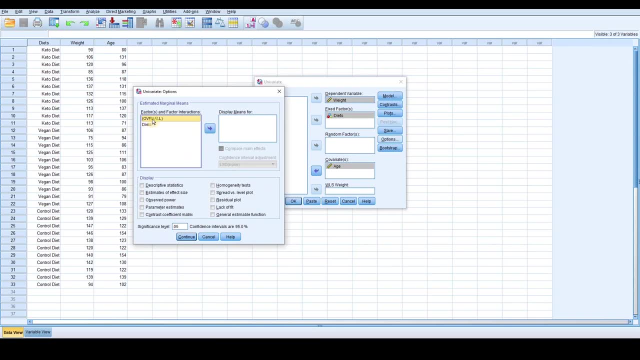 Click continue to close this dialog box. Finally, click on the options button In this dialog box. transfer the two items in the box at the left to the display means box at the right. Then check the box for compare mean inferred and click on the button for confidence interval. 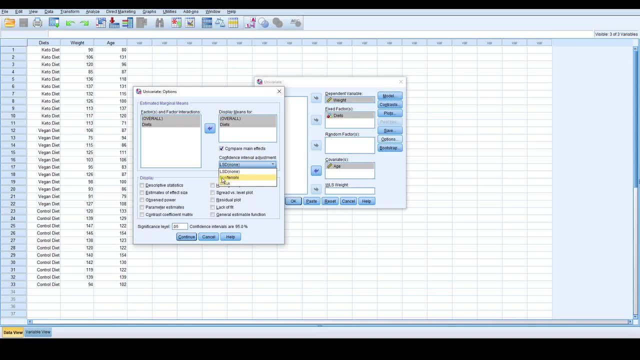 adjustment From the drop-down options. click on Befaroni to select it. Then come down to the display section In this place. click on the display section. In this case, check the box for descriptive statistics to produce the mean and standard. 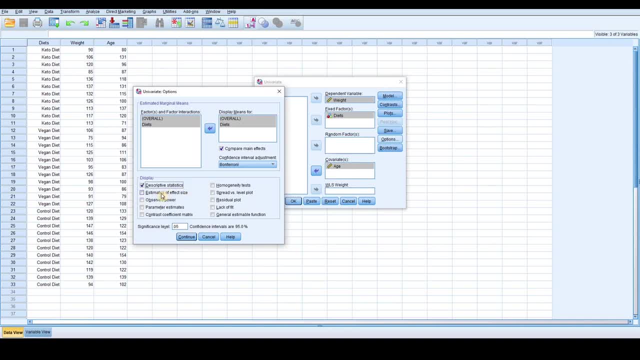 deviation. Check the box for estimates of effect size to give account of the variance explained in percentages. And finally, check the box for homogeneity test to test whether the error variance of the dependent variable is equal across groups. Click continue to close this dialog box. 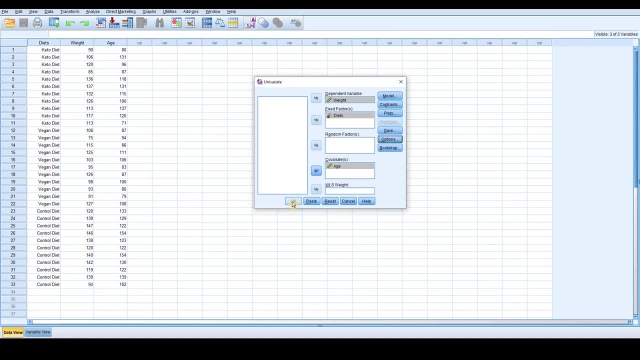 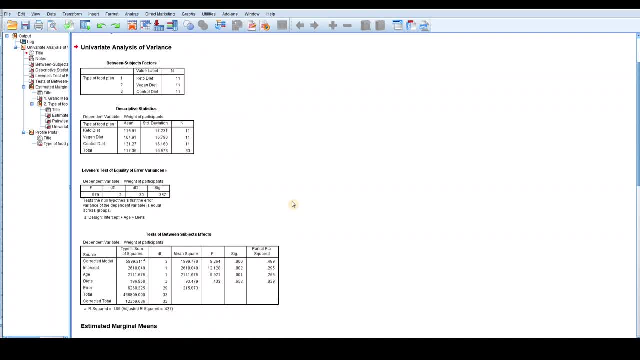 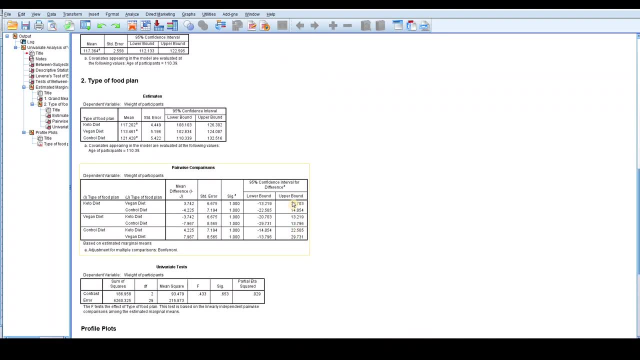 And now click ok to perform the uncover analysis, And you can see that the results are already being produced. Now the next step is to interpret the results. So watch out for the next video, where I will demonstrate how to interpret the uncover analysis.